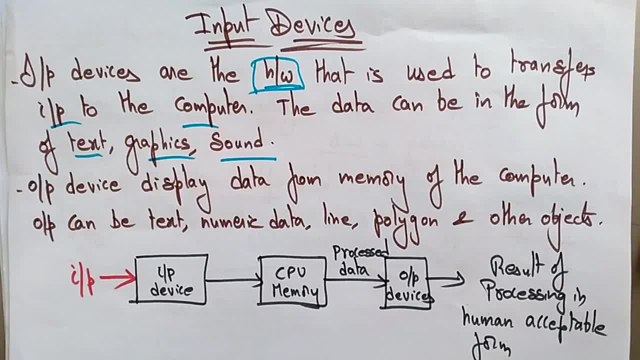 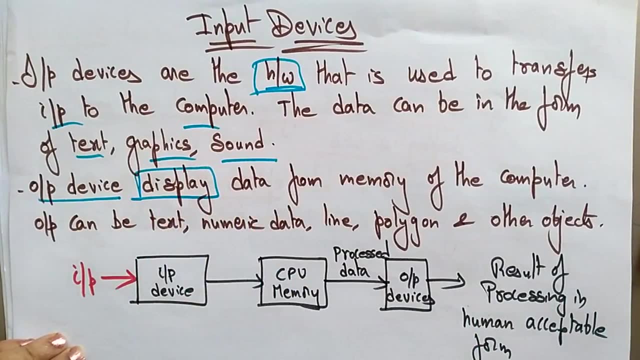 you need to type the user keyboard and the graphics sound microphone. So those are all the input devices And the output devices is a display data from memory to the of the computer. And coming to the output devices, output devices, we call it as a display, So it is what it is going. 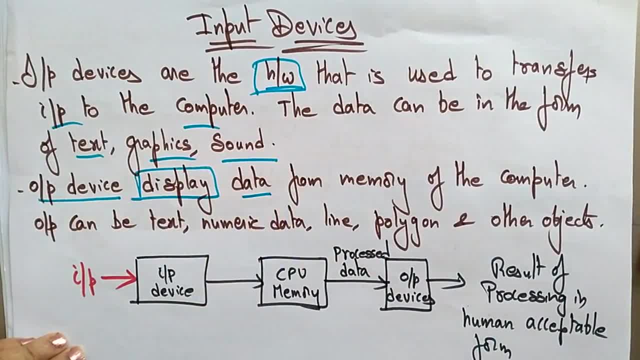 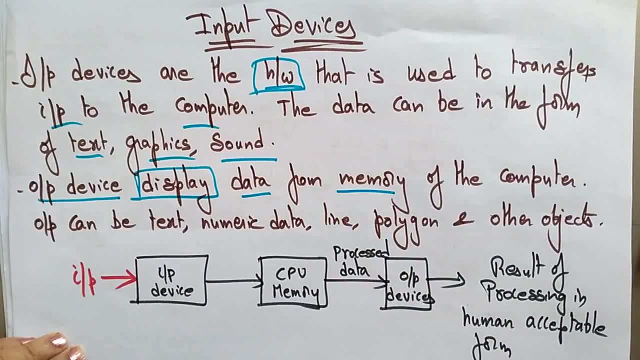 to display. it is going to display the data. So from where it gets the data? from memory in the computer. In the computer you are having the memory. From the memory it takes the data and displays on the screen. So, whatever you are able to see, that is an output. devices, The output. 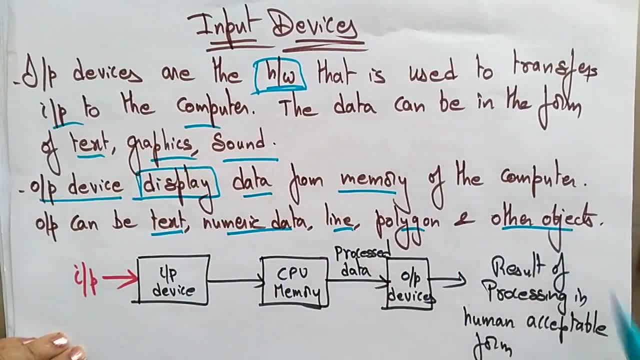 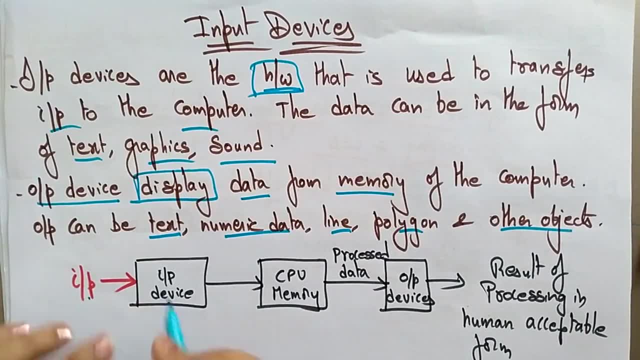 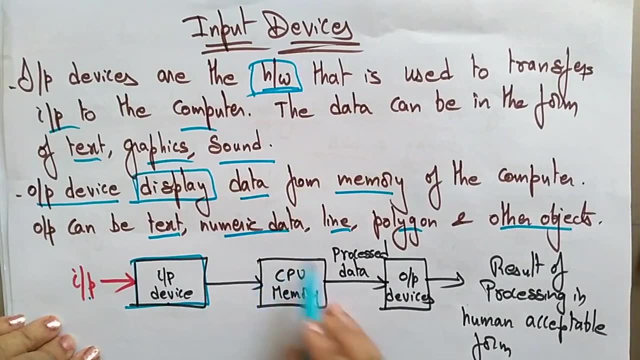 can be a text, numeric, data line, polygon and even the other object also. So input that you are giving, that input is giving with the help of input devices, That input devices sending the information to the CPU and the memory. So after performing the operations, the CPU is going to 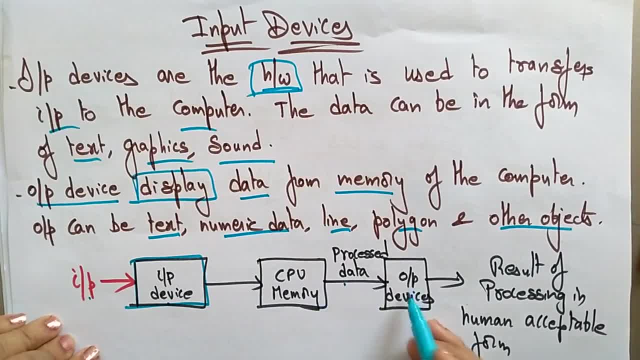 process the data which is taken from the memory and that will be displayed to the output devices. So after, in the output devices, we are getting the output, So that that result of processing the human acceptable form means we the whatever we are able to. 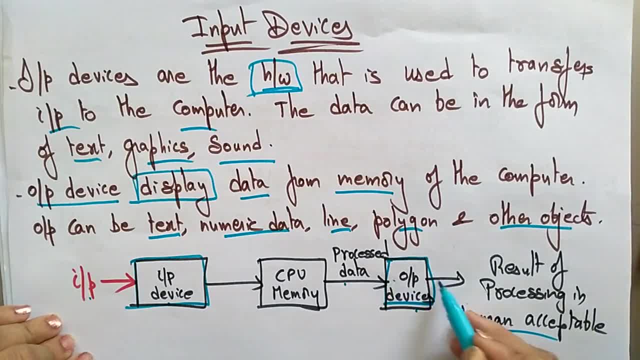 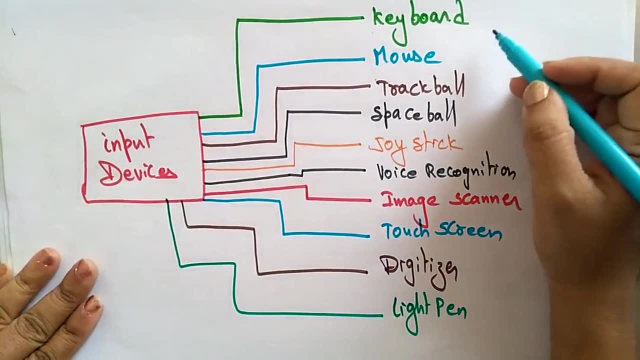 understand In that format the output devices sends the data to the output means as an output. Okay, So this is an input and output. Let me show you some of the input devices. Some of the input devices are the keyboard, mouse, trackball, spaceball, joystick, voice recognition. 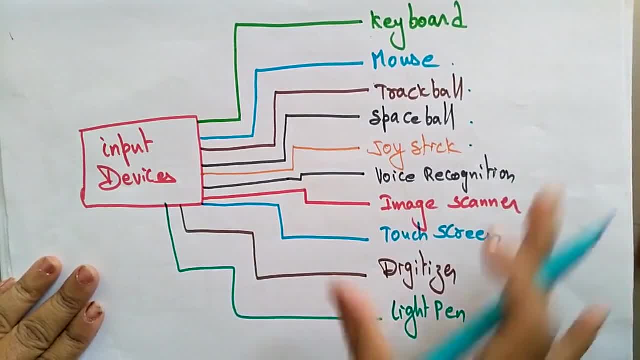 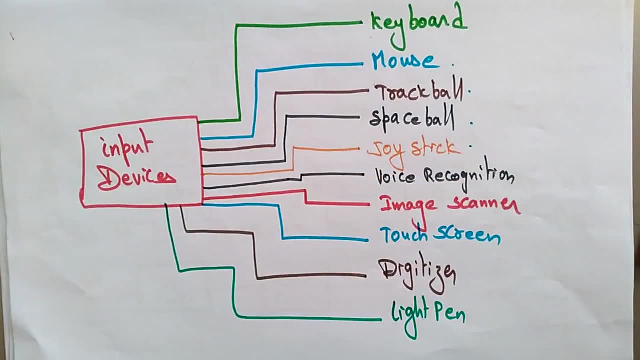 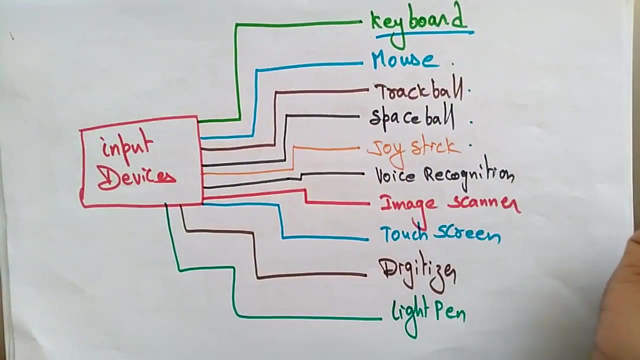 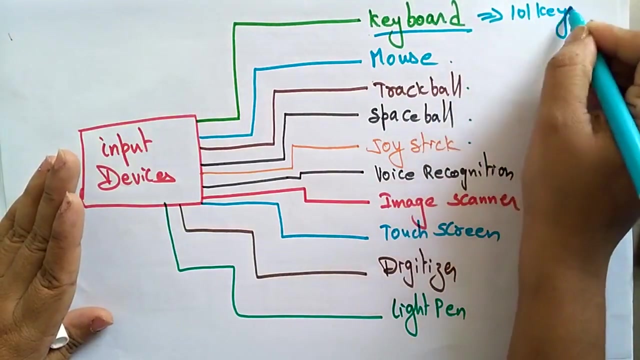 image scanner, Touch screen, digitizer, light paint. I know you all. you already know all these concepts, So just me, let me recall, Okay, A little bit. So what is a keyboard? You already know the keyboard, which is a most common used input devices. It's having a total 101 keys that are present in your 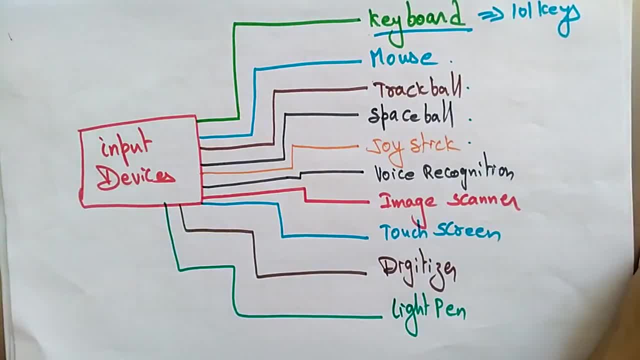 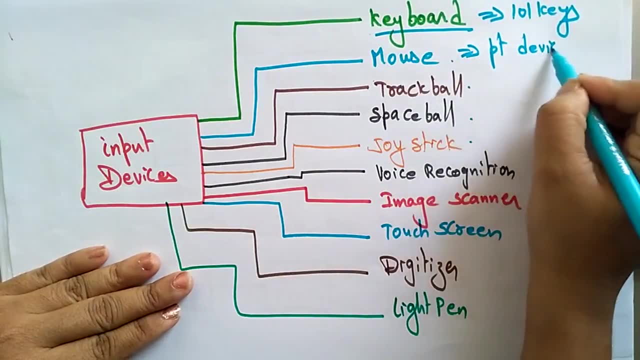 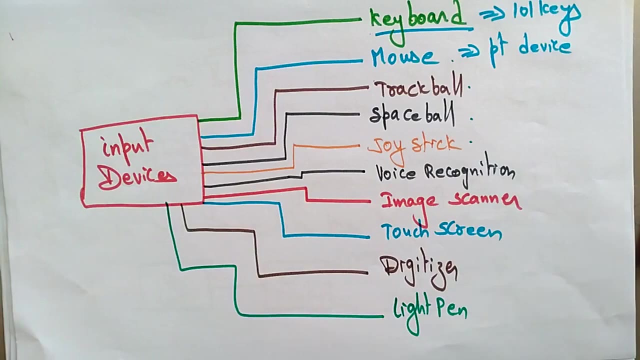 keyboards. Okay, So this is a most common used input devices. And next is a mouse. Mouse is a mouse. You call it as a pointing device. It is pointing device, So, and the one thing that you have to remember that it cannot be used to enter the text, It's just only pointing, It's just a. 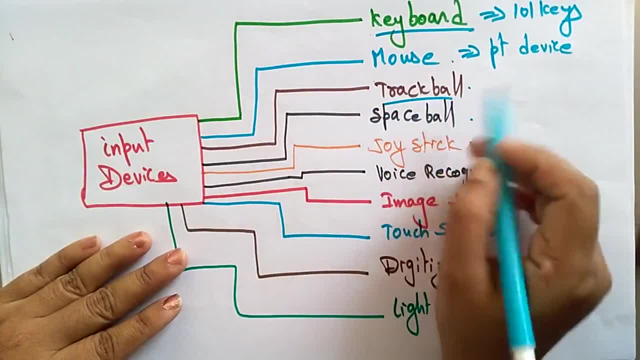 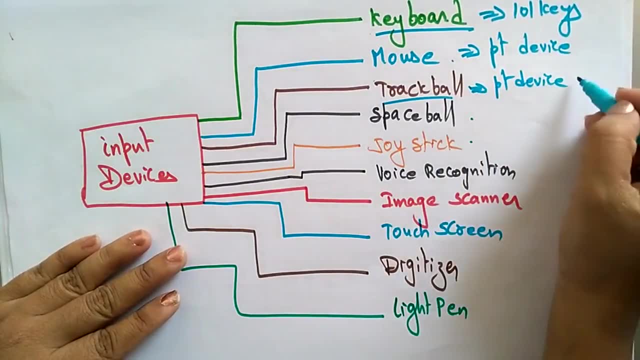 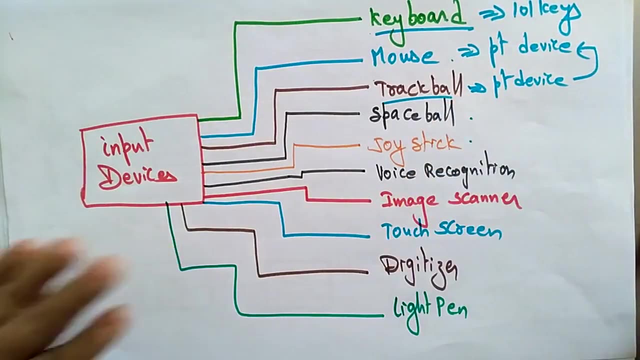 cursor, the pointing device, and the trackball. The trackball is also a pointing devices. It is also a pointing devices similar to the mouse. It's just similar to the mouse, but here this is mainly used in the notebooks or laptop. 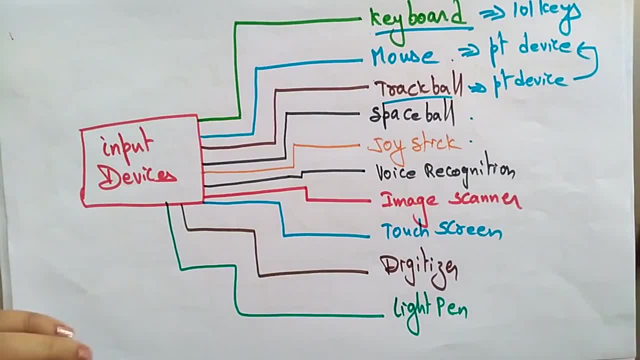 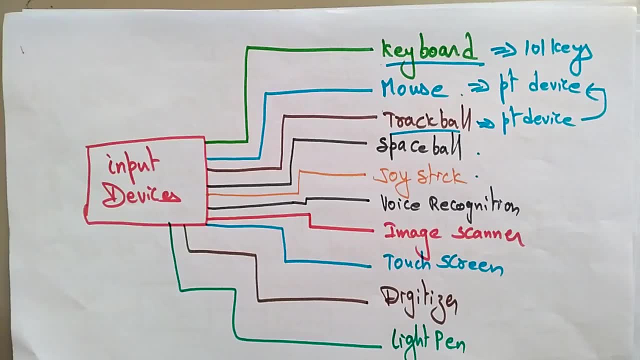 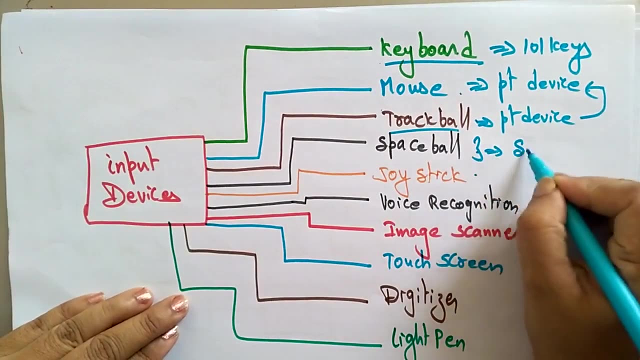 computers instead of the mouse, Suppose. if you don't have instead of the mouse, we can use this trackball. Next is a spaceball. Spaceball is similar to that of trackball, but it can move in six directions. The spaceball can move in six directions, Whereas the trackball is move only in. 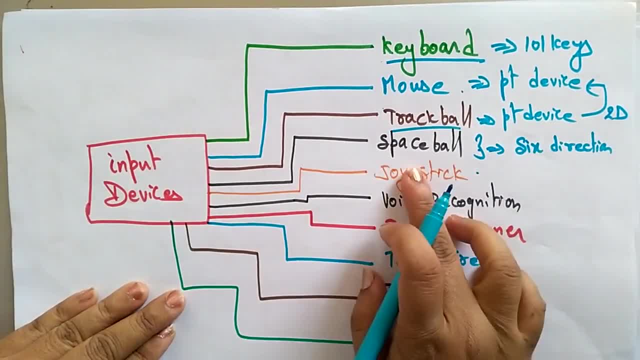 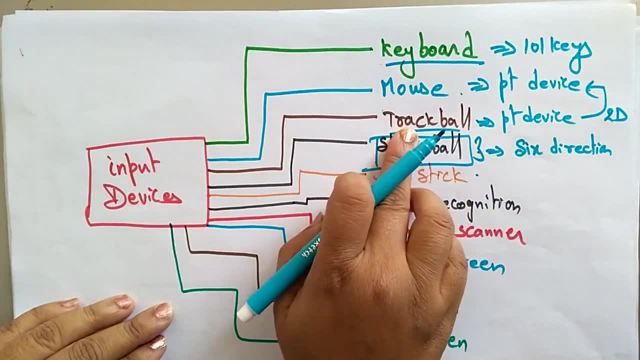 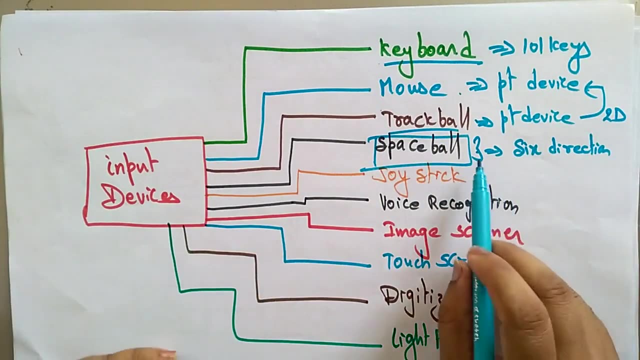 two directions, So it is moving only two directions, but spaceball is moved in six directions. Then, where we use this spaceball- So I said trackball can be used in the notebooks or in laptops instead of the mouse, And where we use this spaceball, This spaceball can be used for 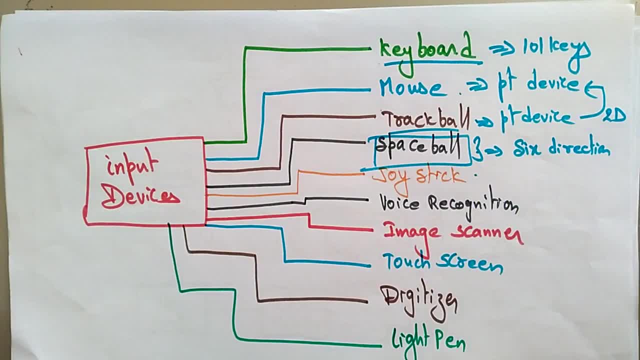 the 3D positioning of objects. In the 3D environment we can use a spaceball because it can move in six directions And it is applicable in the CAD applications, that is, the computer aided design applications, And it is also used in the animations. 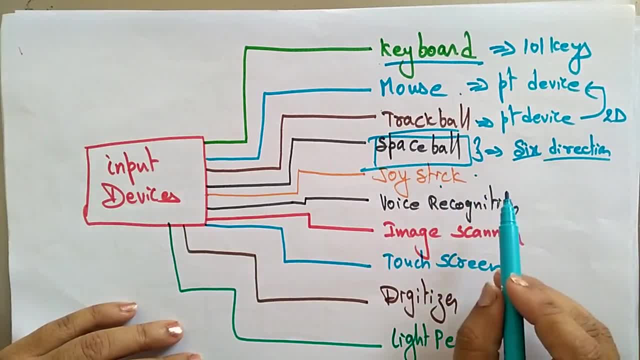 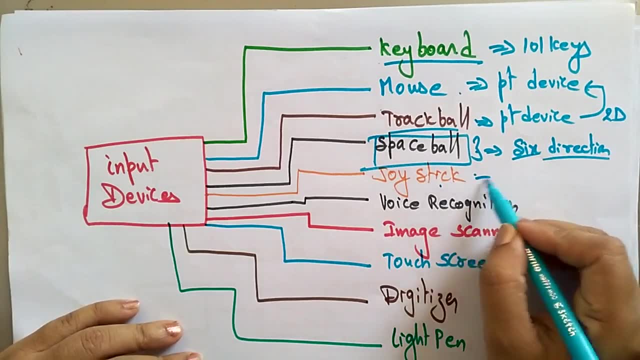 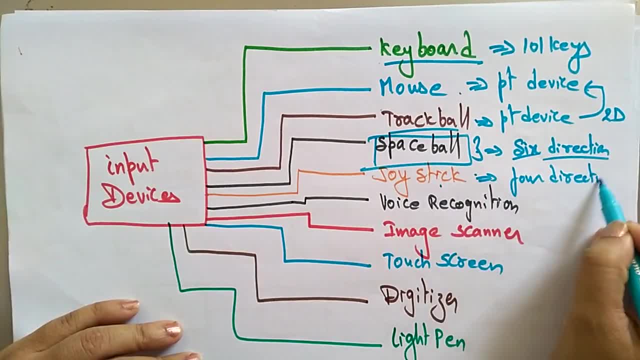 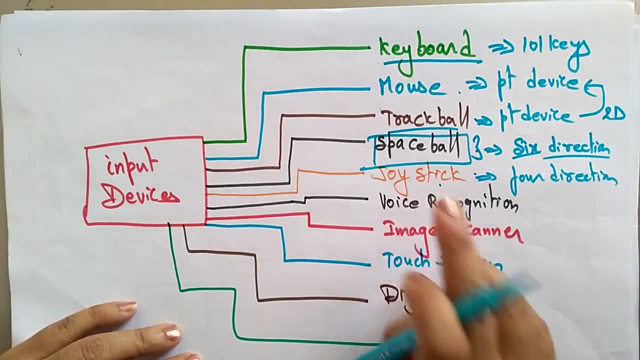 So it will be four directions. A joystick can be used in four directions. Space is six direction and track is only in two directions. And where we use this joystick? The joystick can be used in CAD designing And even in the playing of computer games. you can use the joystick. You know the voice. 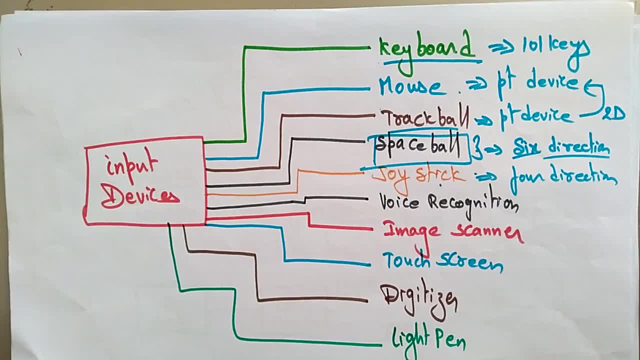 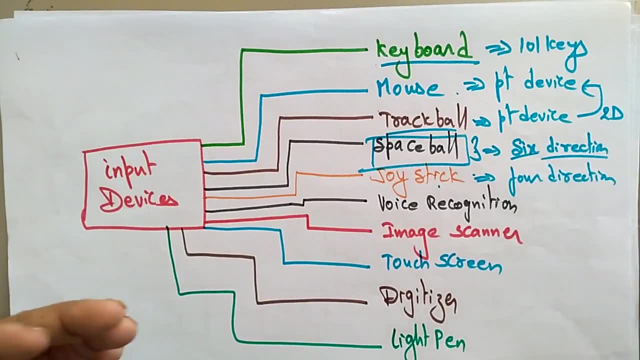 recognition. so with the help of that microphone, the voice can be recognized and it will be perform the operations. image scanner: so what? it will just print this message on the paper. uh, images, or the text, whatever it may be, that can be uh, print on the paper. so you just place that.